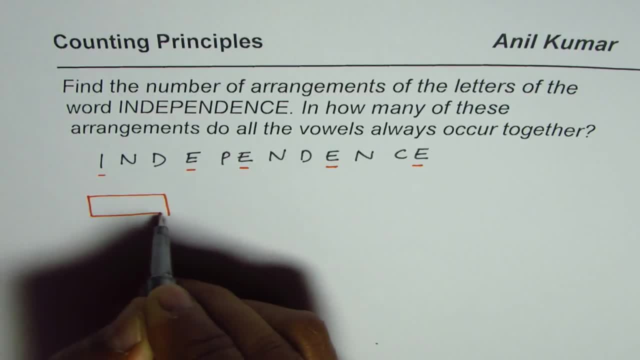 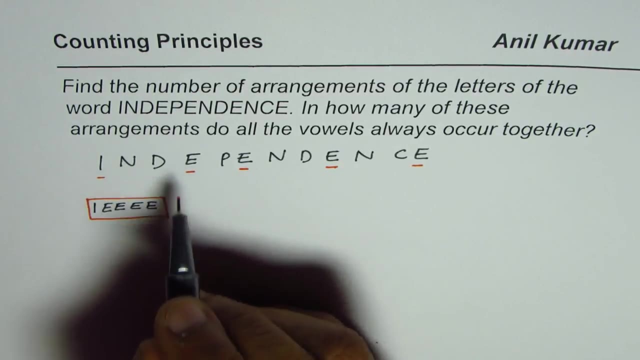 is that we can make a block in which we have one I and four E's And then rest of the numbers. Let us write. So the rest are how many We have one, two, three, four, five, six, seven, eight, nine, ten and one I. So we have one, two, three, four, five. 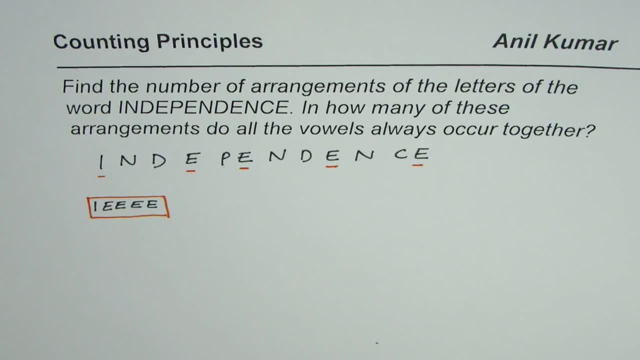 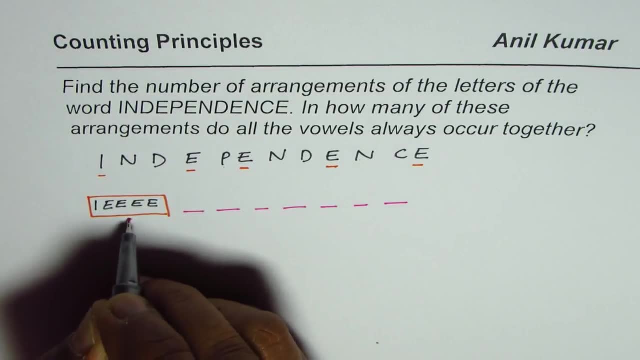 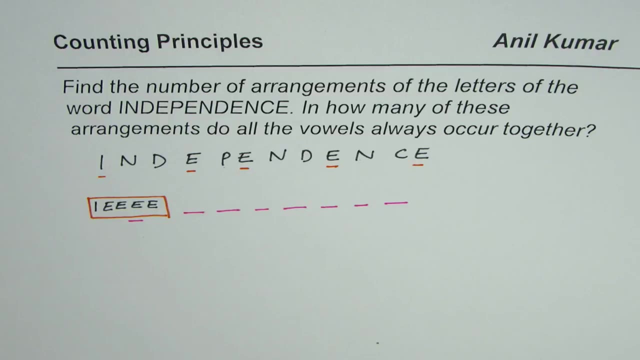 six, seven, right. so we are left with seven others: one, two, three, four, five, six, seven. so in a way we will count this block as one and seven others. so we are left with a combination of these, correct? now you'll notice that in this word there are some letters which are repeated, so they are going to. 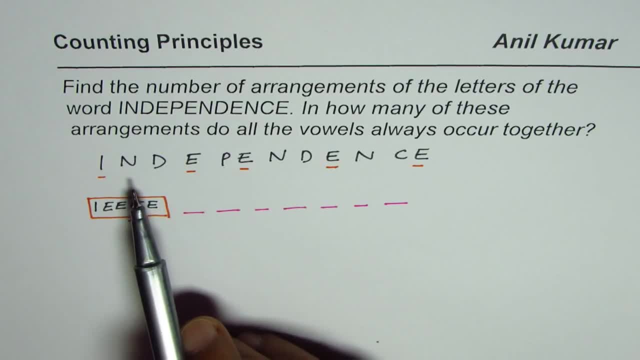 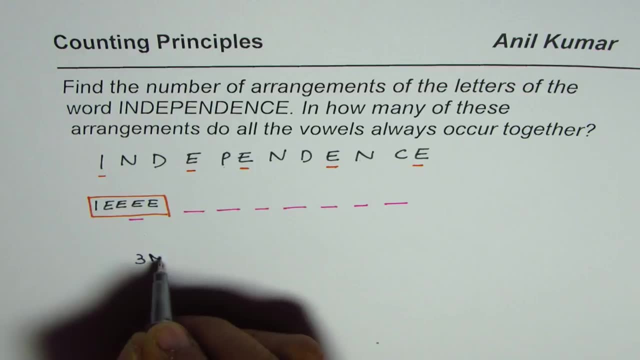 restrict or reduce the number of selections. so how many n's are there? we have three n's. so here we have three n's. okay, so we're taking care of n's. two d's so we have two d's. okay, so no other word is repeating. three n's and two d's, so that is the number of repetitions in the particular group. 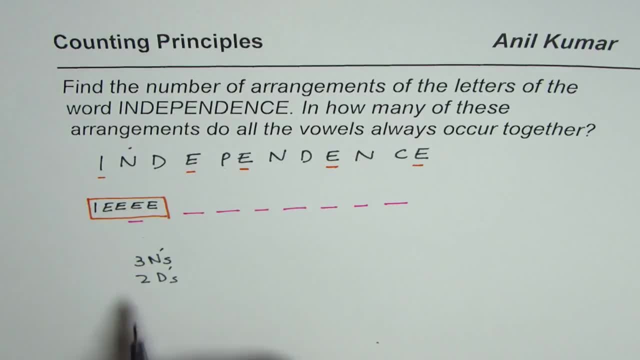 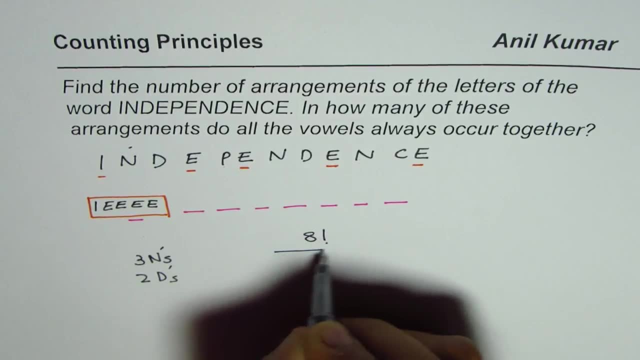 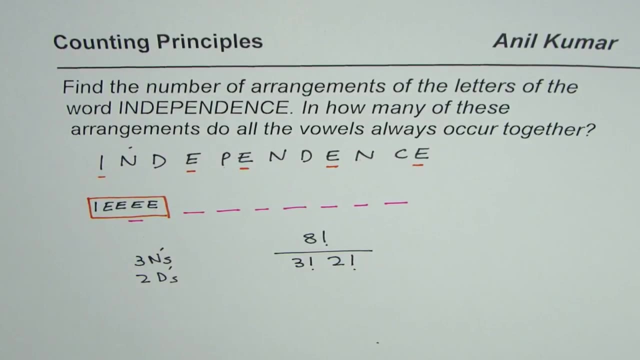 and therefore, since these are repeated, the count should be eight. are the positions. so eight factorial divided by three factorial times two factorial. so whenever you're doing permutations where some are identical- in this case three n's and two d's, we have to divide by them, since our 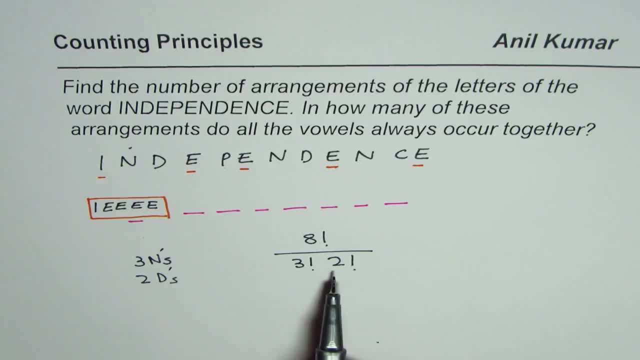 number of selections become lesser by that factor. now, for each of this combination, within this set which we took, set of vowels, they can also be arranged differently. so what we have here is five right. so we have five of these letters which could be arranged, and since there are four e's, so number of ways it could be arranged is five factorial.